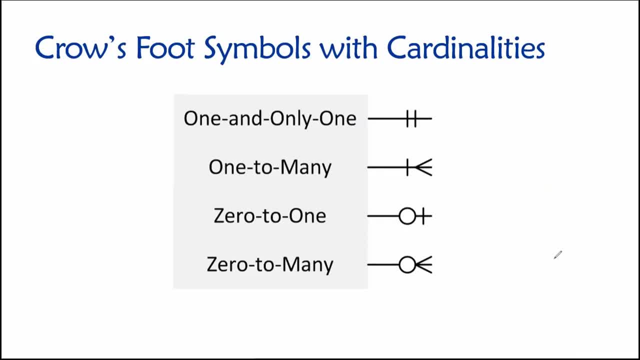 So all you need to do is know those three and that you can interpret any of these line endings that you might see here: Uh, what's not illustrated here Is that, uh, these would be connected to some entity. okay, So maybe that's like a- uh, an employee table, or this one's like a department. 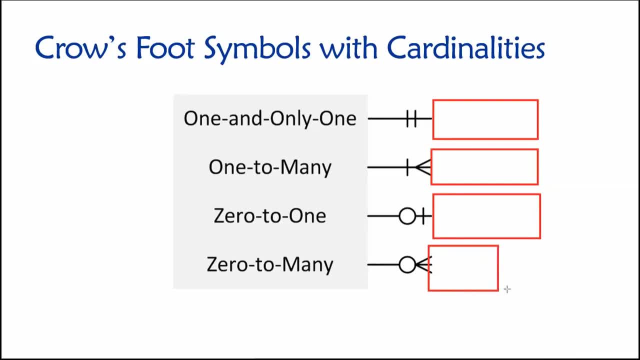 table or a customer table or whatever. So these line ends are going to be connected to some table and they tell us something. We'll use this one here as an example. So imagine that you know, just for the sake of illustration, that this is an employee table. 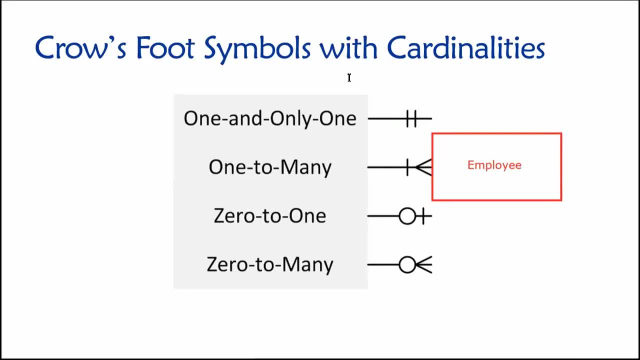 So we have these two symbols, and one of them Is going to tell us about the minimum cardinality and, uh, the other one is going to tell us about the maximum cardinality, right? So in this case, what we need to remember is that the symbol that touches the entity 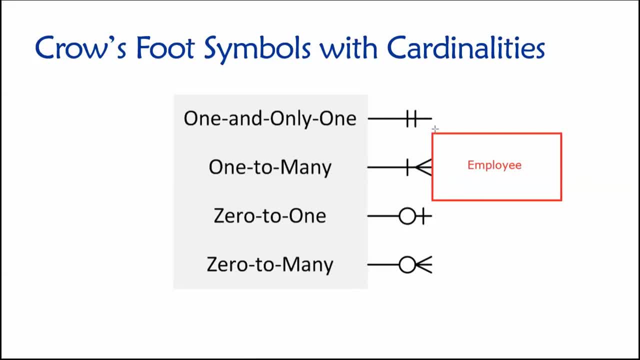 So you can see the symbol here That's touching the entity, where our entity is indicated by this rectangle. Those are the boundaries of the entity. That is the maximum cardinality right, And the one that is not touching the entity is the minimum right. 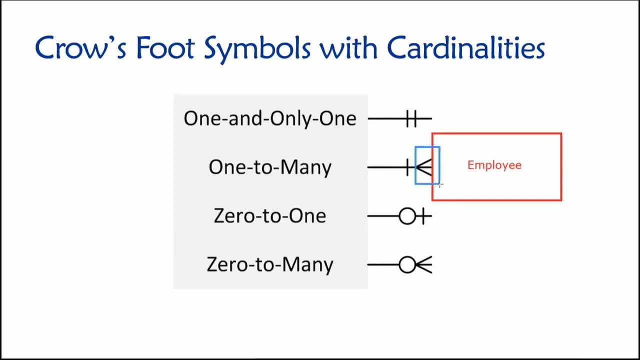 So this represents a minimum cardinality of one and a maximum cardinality of many. That's why we describe it as a one to many relationship. Okay, So here's a zero to one right. Here's a zero to many. Here's a one and only one, or a mandatory one. 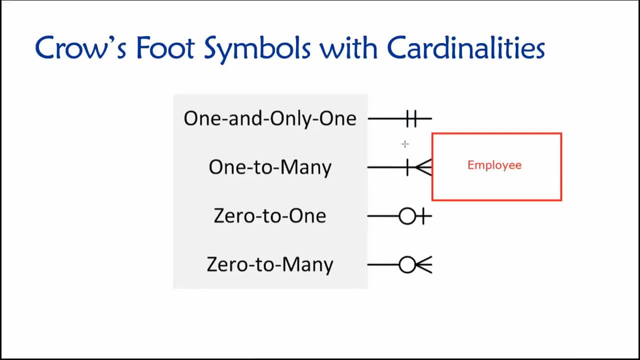 Or exactly one, whichever you prefer, Hmm. So let's build out these concepts a little bit and see if we can learn to interpret some of these diagrams. Now, what we see illustrated here is these symbols flowing in one way, That is, they're oriented only in one way. but we need to develop the mental flexibility to read. 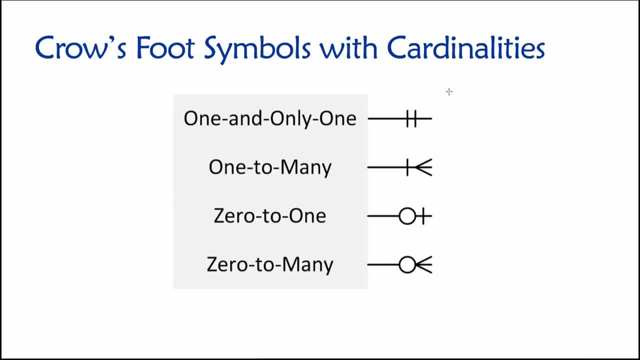 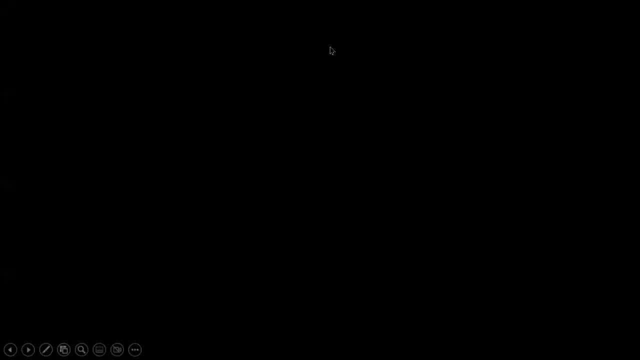 these minimum and maximum cardinalities, Regardless of the orientation in which these relationship lines and symbols have been drawn. So I will happily illustrate what I'm talking about with some lovely tables. So let's imagine that. no, we have some tables that are related to each other here. 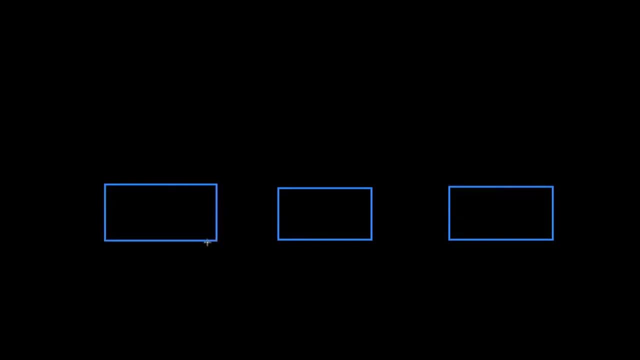 I'll just draw some various tables. We'll do five of them so that we can have a complete illustrative example. So just imagine that each of these is a table, Okay, And we're going to have some relationship lines that interconnect naturally. 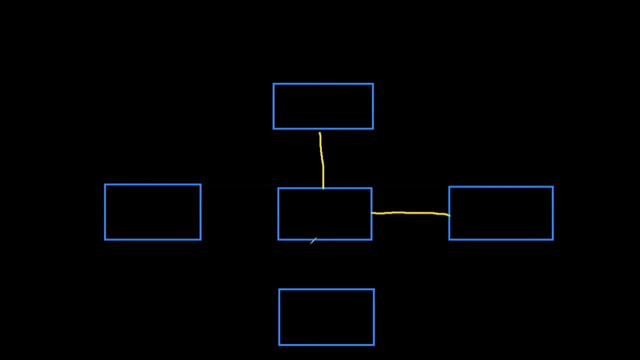 So what we saw illustrated on the previous slide would be something that looks like this: All right, But we need to have the mental flexibility to see that, regardless of rotation, So regardless of the orientation in which we might draw something Okay, We need to be able to read that relationship. 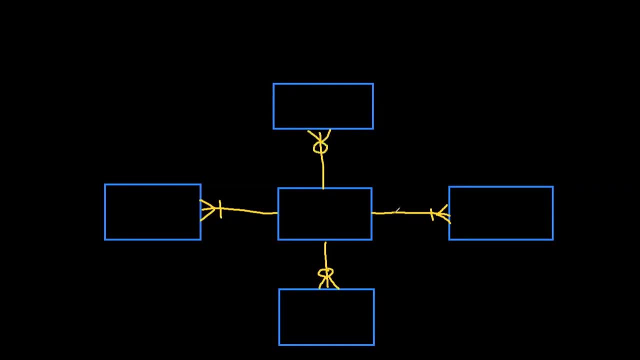 I'm just drawing some examples up here, And of course we would have symbols on the other side as well, And I'll just draw a variety of them for the sake of allowing your minds to figure this stuff out. So on the previous slide we saw things did horizontally. 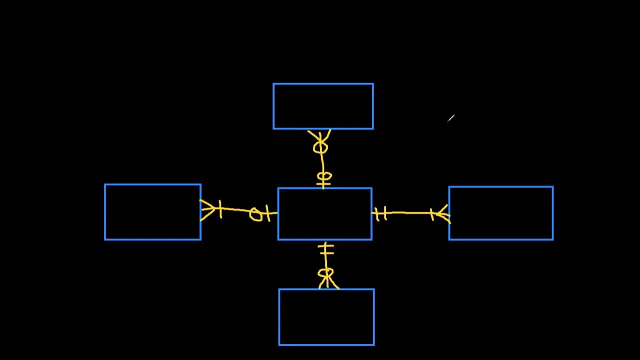 But, as we see here, that was just one of several possibilities. right, We need to be able to have the mental flexibility- Flexibility to rotate these things in our minds and still read it. Okay, So if I just fill in some values here for the sake of being able to describe things, let's say that this is, I don't know, a table. 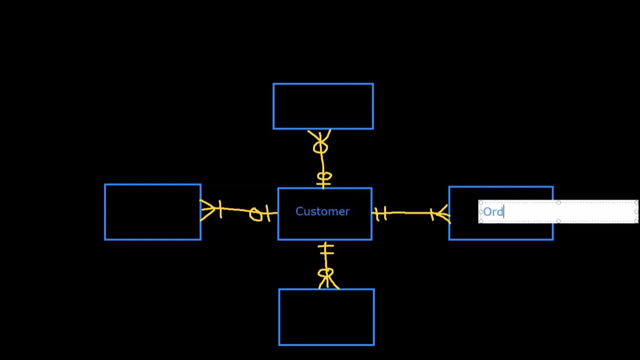 And this one over here is an order table. So what does this say? How can we read this relationship? I don't remember. We read these relationships in two directions. So if I'm reading it in the direction from customer to order, This direction, customer to order- 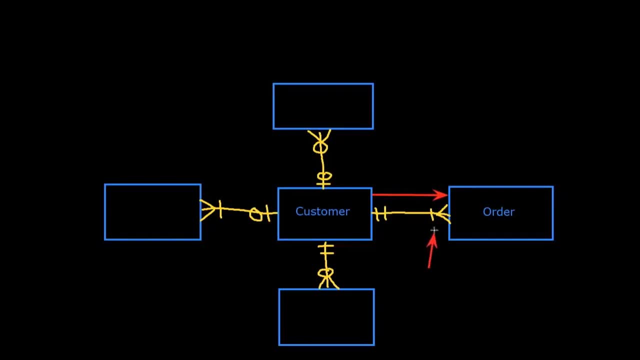 I would say: each customer places one to many orders, right. So this is a one to many relationship in that direction. Each customer places one to many orders, which makes sense, right? Because someone can't be your customer unless they've ordered something from you. 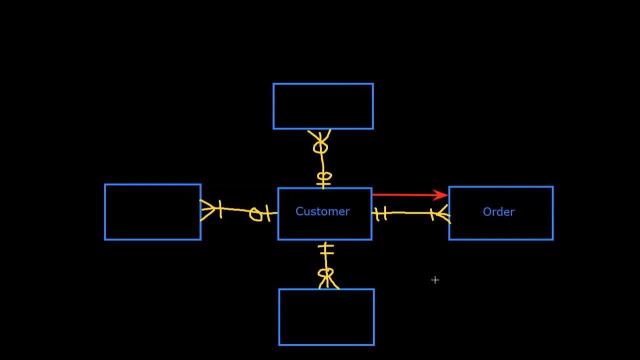 Am I really a customer If I just walk into a store and walk back out I don't know, I didn't buy anything. So, who knows? this gets to the semantic definition of what is a customer. It's a philosophy. Now, if we took a look at the same relationship in the opposite direction, 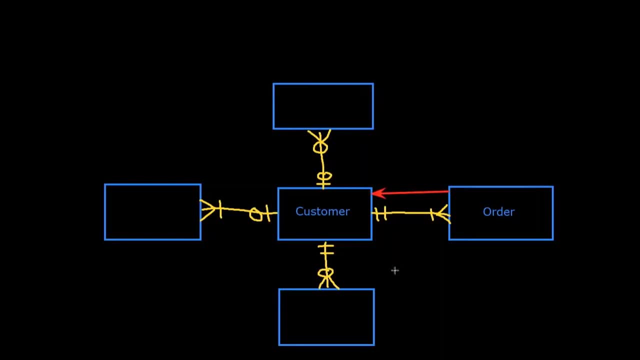 that is in the direction from order to customer. we would read it as each order is placed by one and only one customer. So the minimum cardinality in that direction is one and the maximum cardinality is one. Okay, Interesting. So we have to have the mental flexibility to read these relationships both. 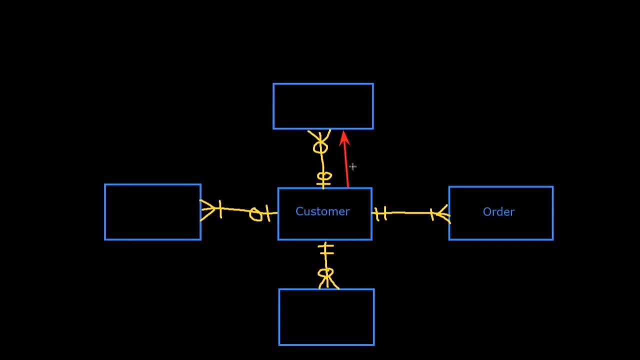 directions, regardless of the way that the lines and the symbols are rotated. If we have some other concept illustrated here, I don't know what I want to call this. maybe this is, since I can't think of anything- entity say: what is the. 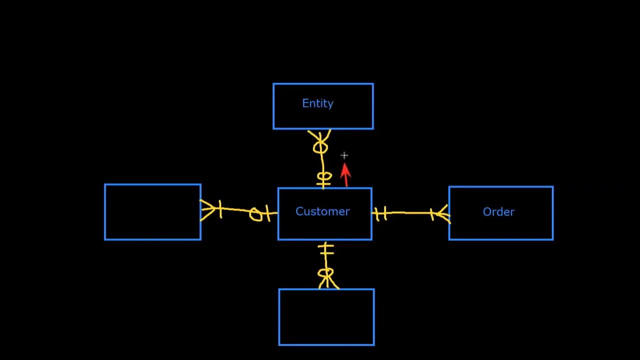 relationship between customer and entity. So in this case, reading it This Direction, we would say: each customer can have zero to many entities. whatever that is, and reading it in this direction, we will say each entity is associated with zero to one customers, right. 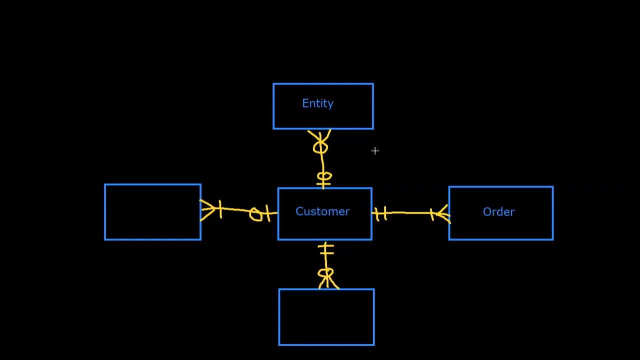 So the minimum cardinality here is zero. Maximum cardinality is one minimum cardinality. There is zero maximum cardinality is many minimum cardinality, zero minimum cardinality, one minimum cardinality, one minimum zero set. So you will notice, looking. 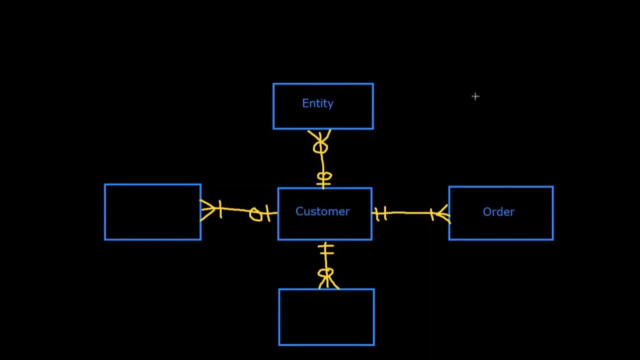 Out here at these possibilities. actually, let me well. no, this is fine. If you look at all these possible combinations of minimum and maximum cardinalities, note the following: the many symbol can only appear as a maximum cardinality, okay, and the zero symbol can only appear as a minimum cardinality, right. 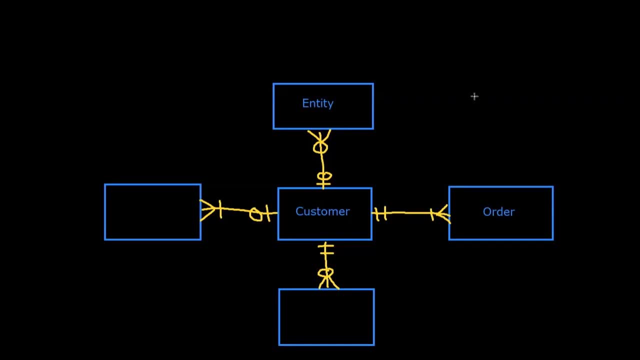 It doesn't make sense to have a maximum cardinality of zero, because that means the maximum number Of rows that can participate in the relationship with another table is zero. So there's no relationship, right If I say that to? the maximum number of connections is zero. 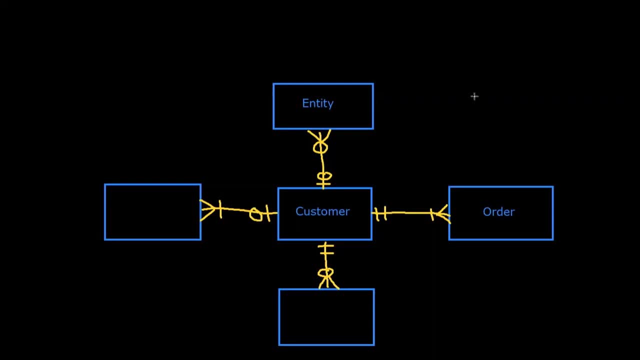 Well then, they're not related. Similarly, I cannot say that the minimum cardinality is many right, It has to be zero or one. So interesting things. clear that out and return back to our slides. So again, just three symbols. 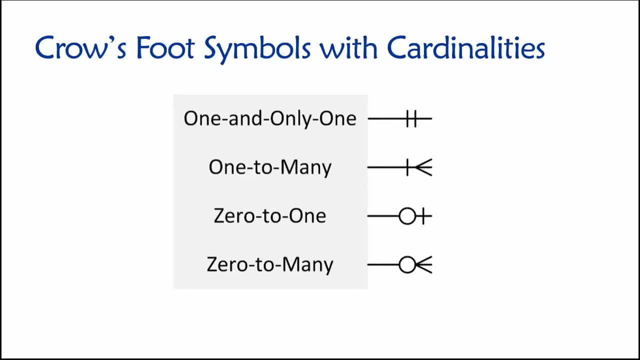 One symbol indicates the concept of zero, One symbol indicates the concept of one And the third symbol indicates the concept of many. with those We can create these four possibilities, And these are the only four possibilities that we use for minimum, maximum cardinalities, to convey information about the nature of the relationship between two. 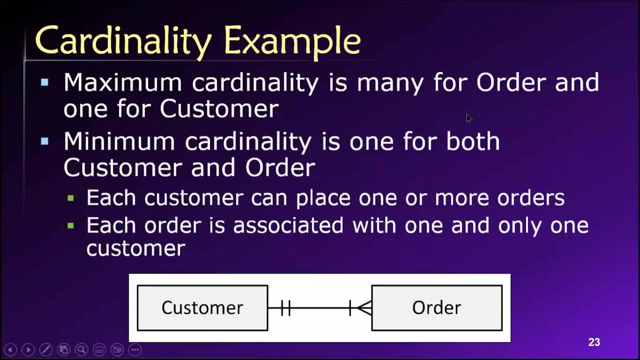 tables in our database. design Cool. So let's take a look at some additional ones here, now that we have the knowledge and understanding of what all these various symbols mean. So here we see a relationship between a customer and an order, And this is very similar to what I illustrated just a moment ago. 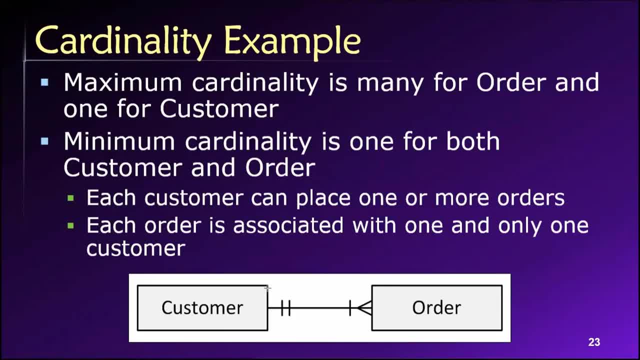 This tells us, when we read the relationship in this case from left to right, in the direction from customer to order, that each customer places one to many orders- Minimum cardinality is one, maximum cardinality is many. If we take a look at that same relationship in the opposite direction, 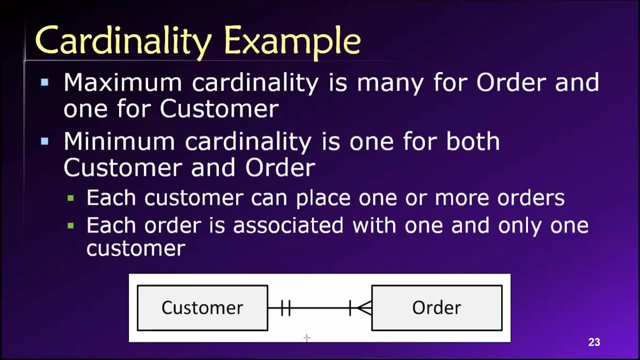 the direction from order to customer. we say each order is placed by one and only one customer. that is, an order cannot exist unless it is associated with a customer. That's the minimum cardinality and each order cannot be associated with more than one customer right. 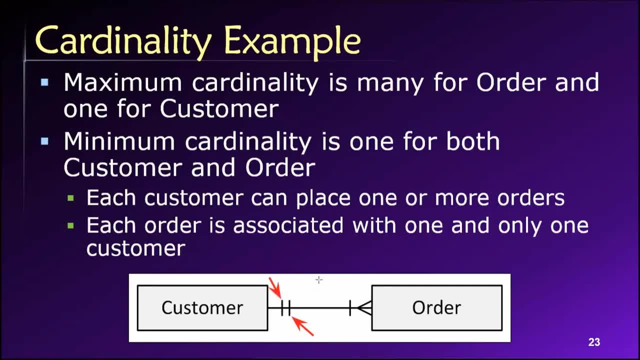 That's the maximum cardinality. So this tells us something about the way that this business operates right. In order for an order to be placed, or In order to exist, it must be linked to exactly one customer, no more and no fewer. 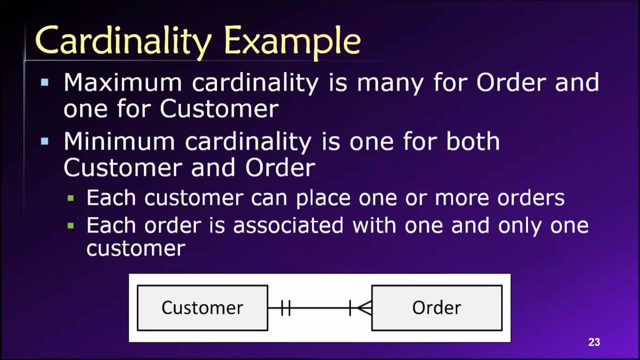 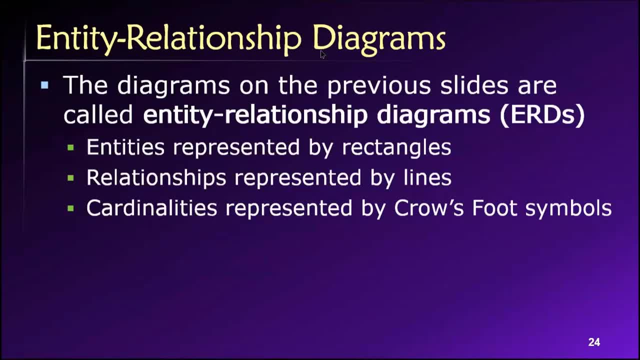 So what we've been seeing here, these types of diagrams, the ones that I illustrated a moment ago. these are entity relationship diagrams, or R diagrams, or ERDs. right, Just different words for the same thing. I like to call them ERDs because it's fast, but I know we get stuck in this world of too many act. 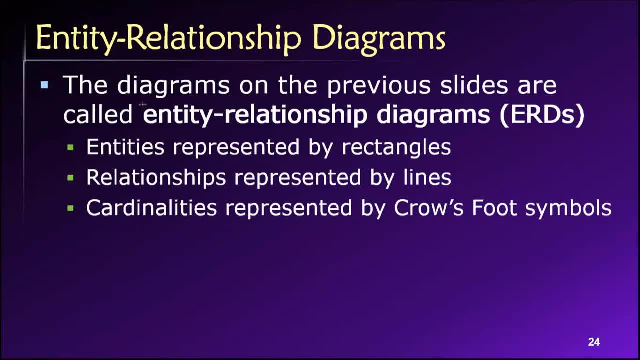 acronyms, So you can call it an ER diagram, an ERD, an entity relationship diagram. It's all the same thing. But just to summarize and revisit, in this world we represent entities with rectangles. we use lines to represent relationships between entities and we.